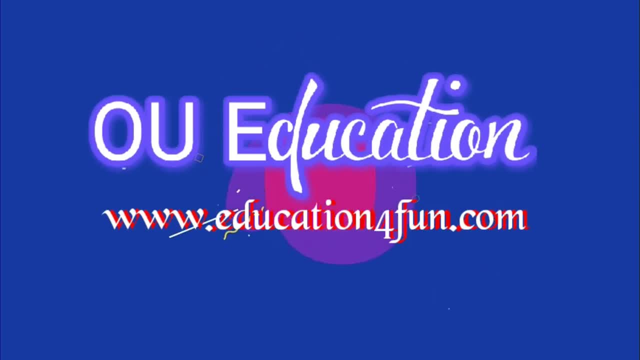 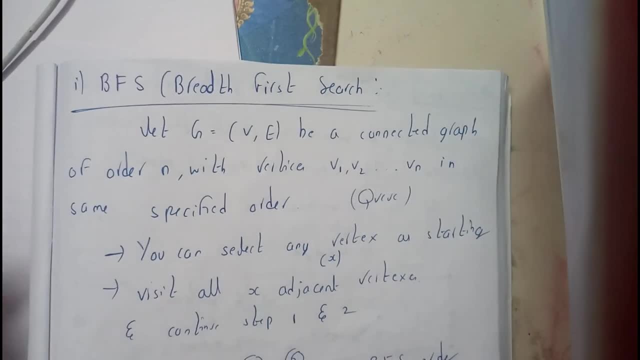 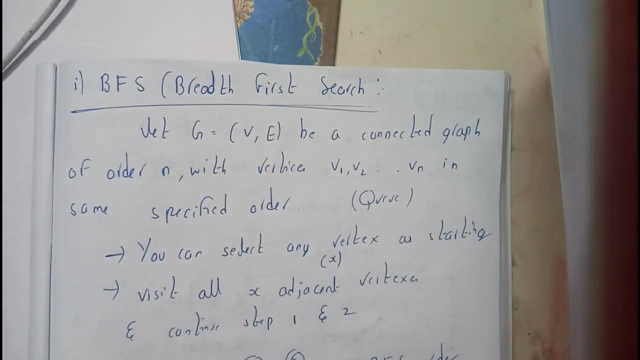 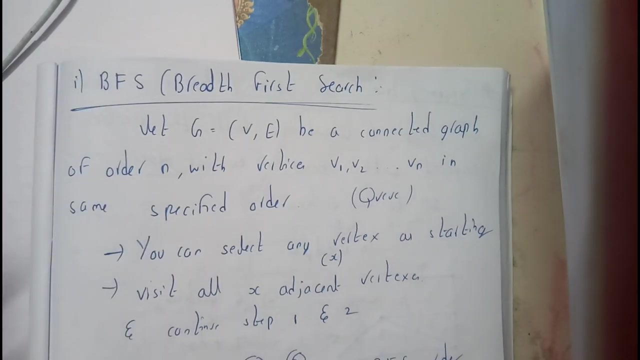 Hello guys, in this tutorial let's see the searching techniques. These searching techniques are majorly used in different, different languages. like we'll be using these in data structures As if this is the breadth first search, This is one of the common searching technique. 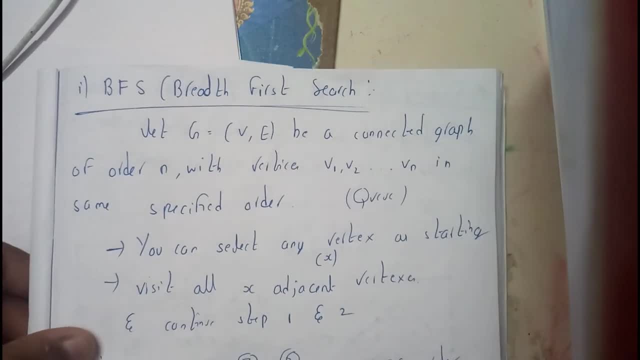 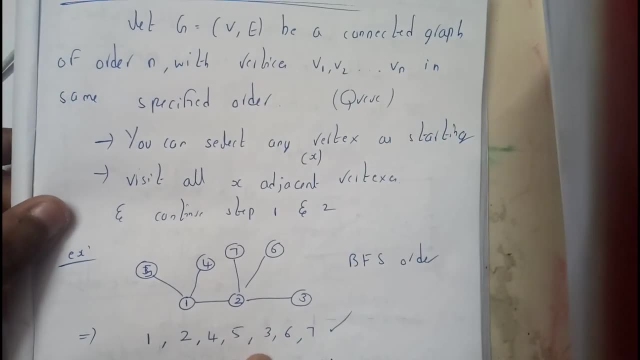 To search an element in a tree. this is a basic method to find Ok. initially, these are the steps. Once we have gone through the steps, I'll be teaching you through an example From the example. it is really easy to understand these techniques. According to the example. 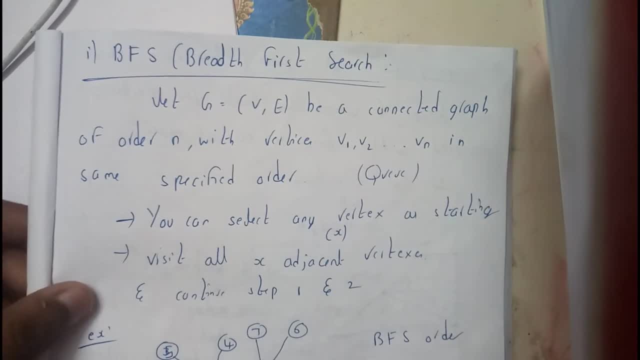 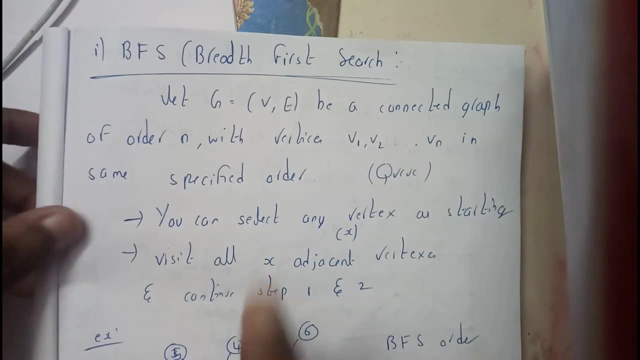 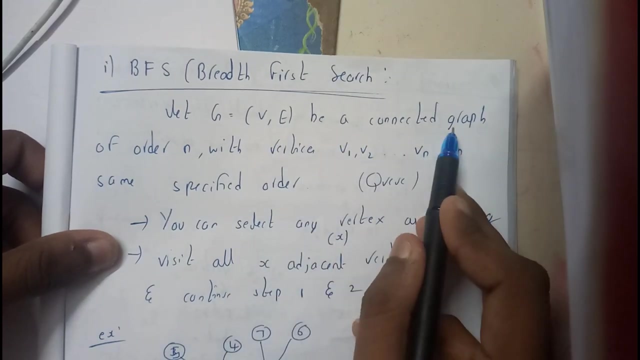 you can just write down the steps as in your own words: Let's go through the steps and then through the example. then I'll be dictating the steps with my own words. Let's see: Ok, Let g be a reference graph. G is a set of vertices and set of edges. be a connected graph if it is a. 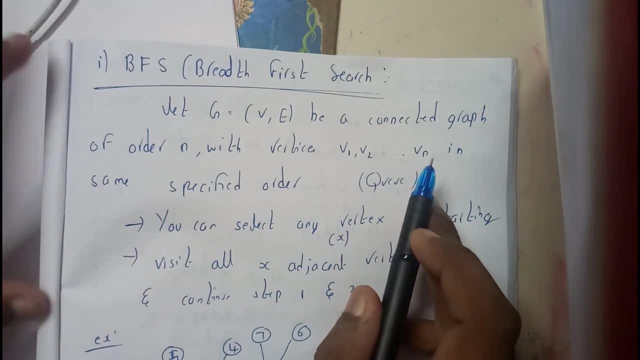 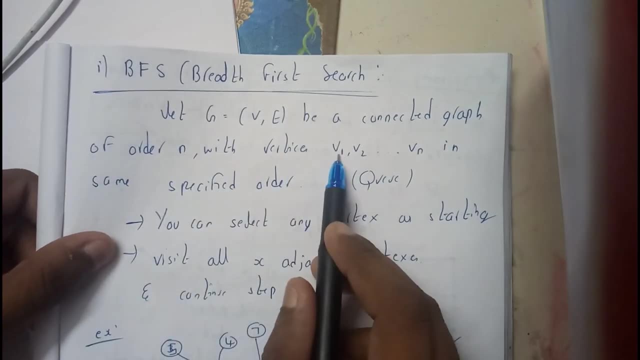 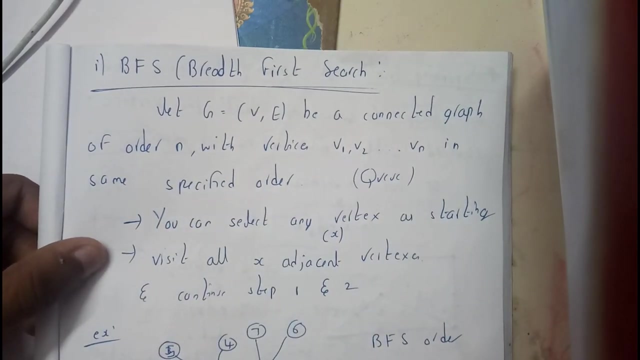 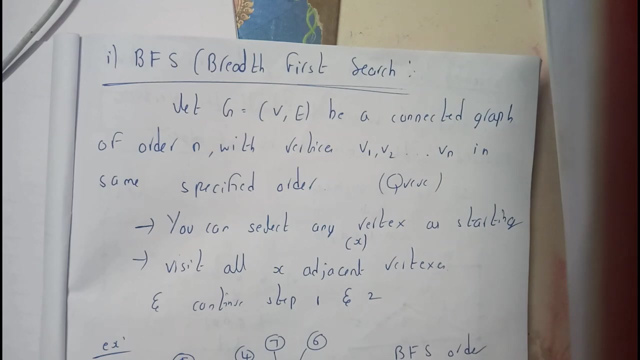 non-connected graph, there is no possibility to search breadth first search or depth first search. okay, that's fine. of order n n be the number of vertices from V 1 to V n in a specific order. BFS is always stored in terms of queues. okay, that's fine. when now we come, whenever we go to the next step, you will. 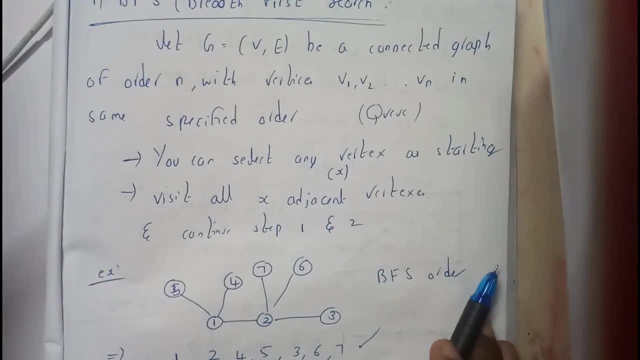 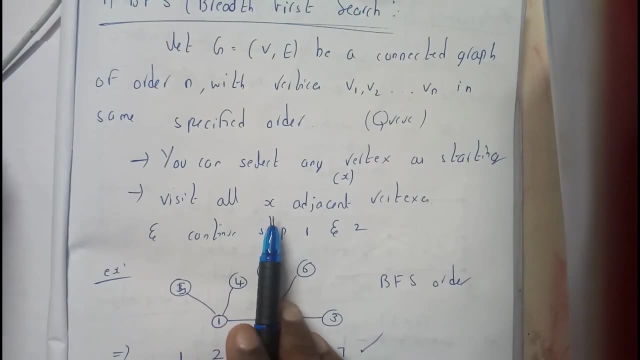 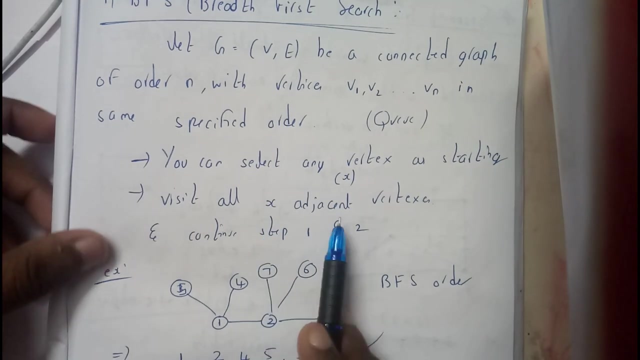 be selecting any vertex as a starting vertex. it's all up to you, it's your decision, guys. okay, that's fine. next, you will be visiting all the adjacent vertices to that, to that vertex, and you will be writing them in the ascending orders. okay, I didn't write it here. okay, that's fine, and you will be writing them. 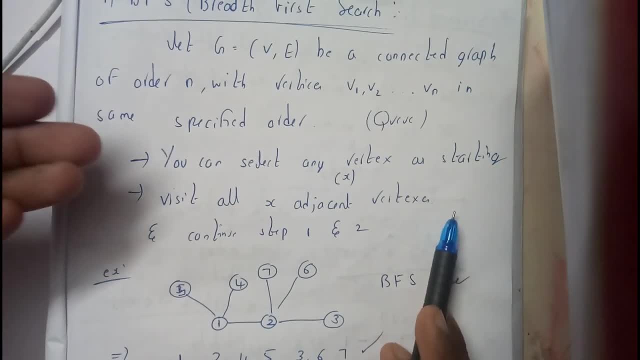 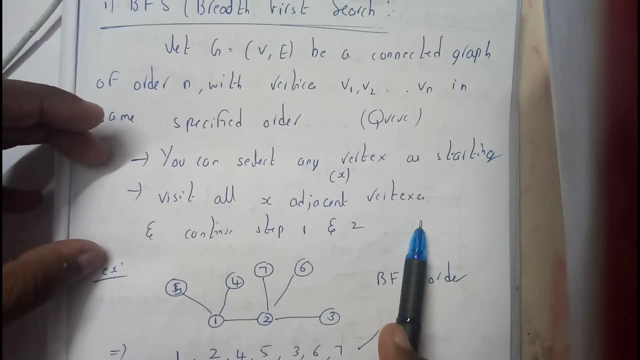 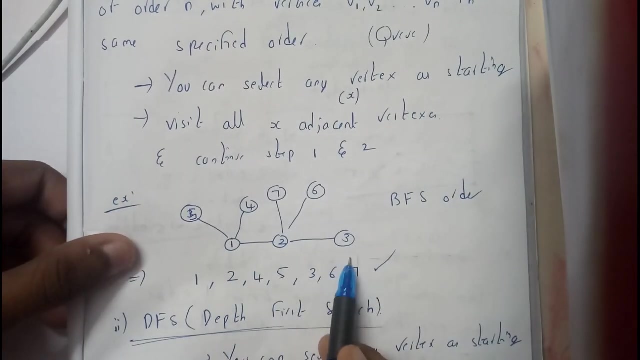 in the ascending order and you will be continuing the same way- steps above step 1 and step 2- and you'll be selecting the next vertex from that pair as the starting vertex and continue continuing it. okay, that's fine. now this is an example. this is a graph, so I have just- sorry, this is a tree, this is a tree. 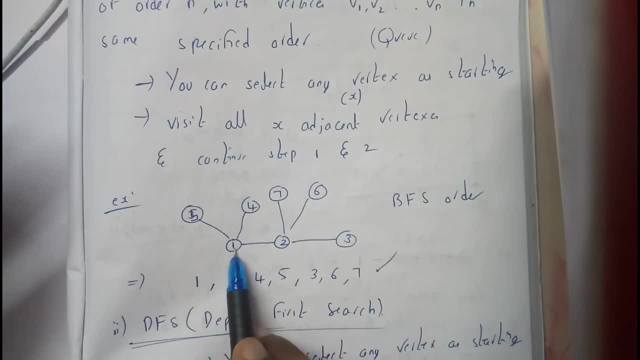 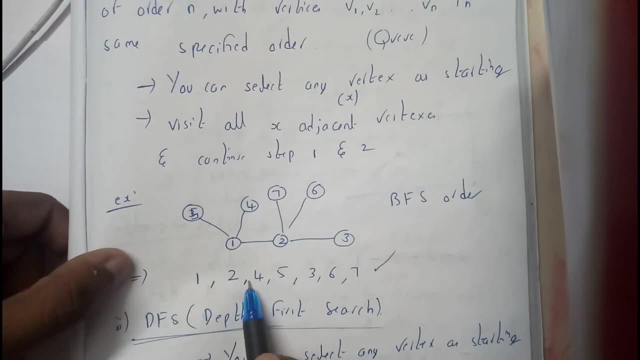 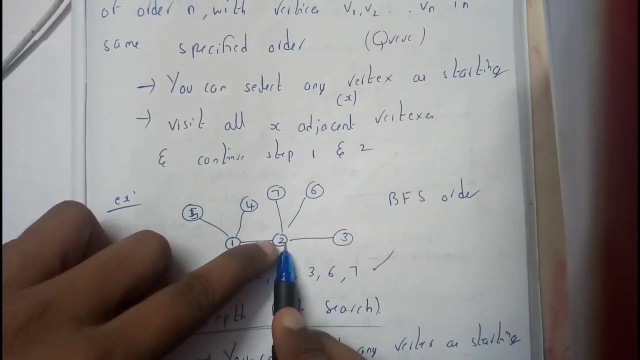 so now I have just took one as the starting vertex, so for this, adjacent vertices are 2, 4, 5. ascending order is 2, 4, 5. right: 1, 2, 4, 5, and now I'll be selecting 2 and I'll be starting its adjacent vertex. 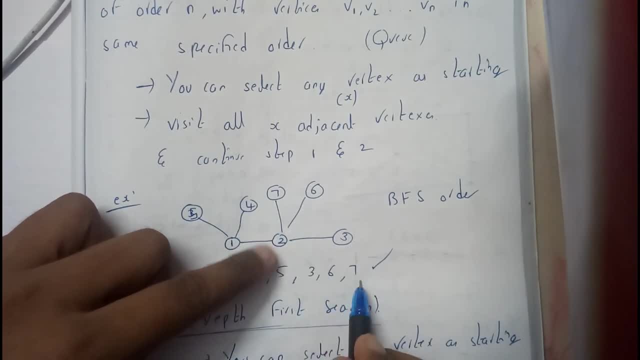 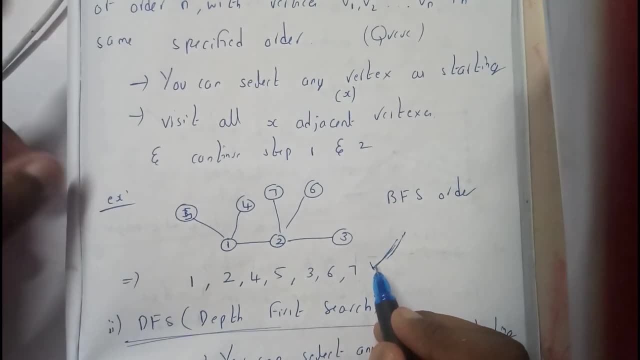 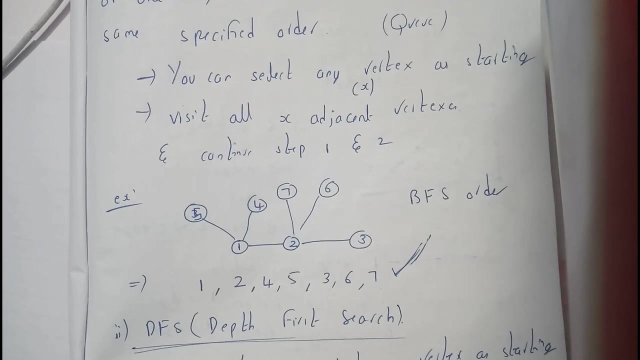 3, 6, 7. ascending order: 3, 6, 7. fine, I have reached all the vertices. hence, this is the breadth first search order of this spanning tree. ok, I hope everyone, every one of you, got this. what a small idea. okay, in my own words, it is clear that I 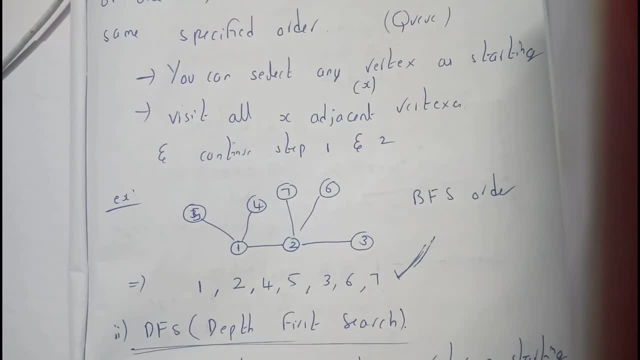 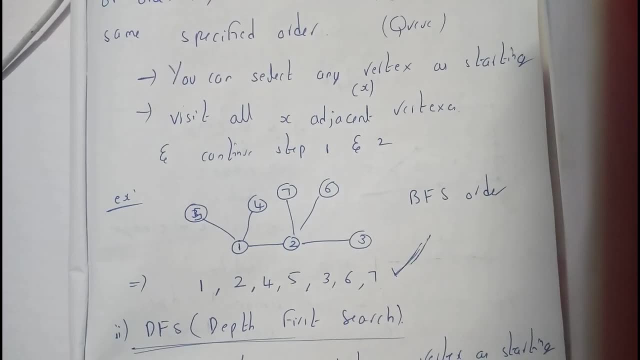 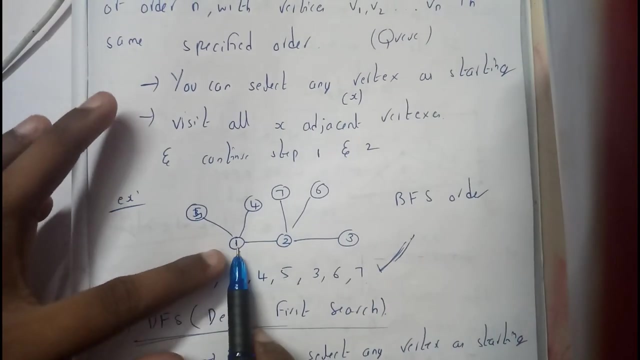 We will be taking a graph G, which has a set of vertices and set of edges of order n. Let the vertices be from v1 to vn and the order is specified particularly in terms of q. Initially we will be selecting a starting vertex, we assumed it as 1, and we will be writing its adjacent vertices in ascending order. 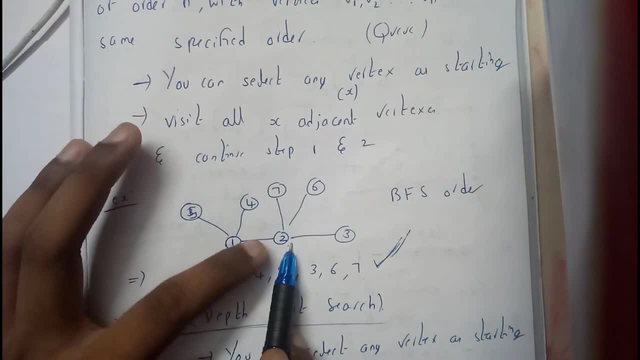 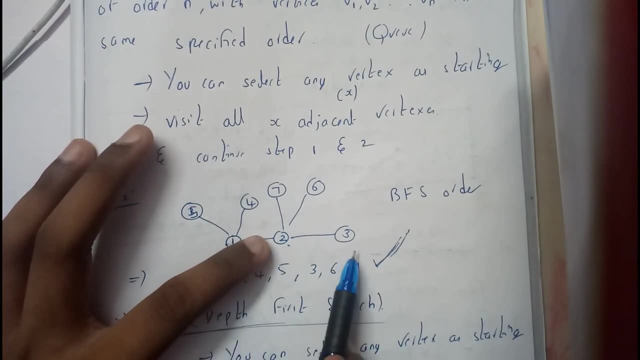 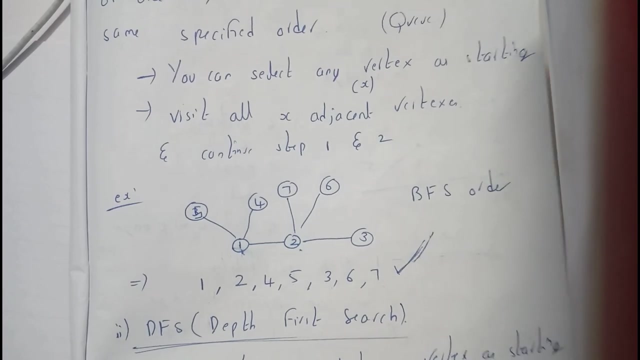 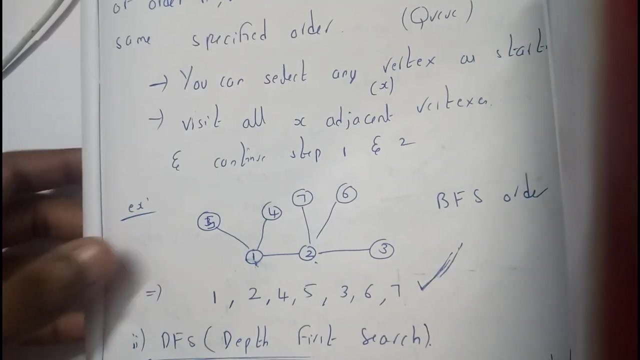 and continuing to the previous adjacent vertex, to the next vertex and continuing it further. on these steps, you are going to get an order such that you visited each and every vertex once. That will be the breadth first search of the given graph. This will be the first part of searching techniques and the second part is depth first search. 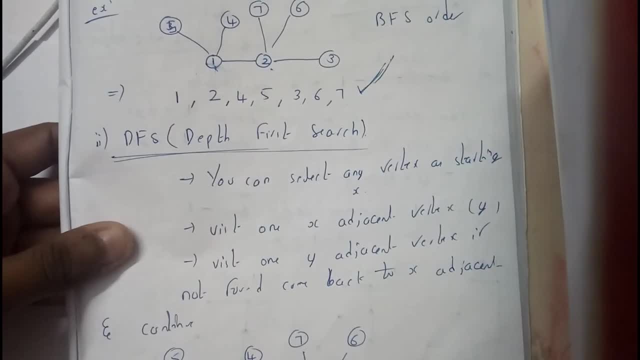 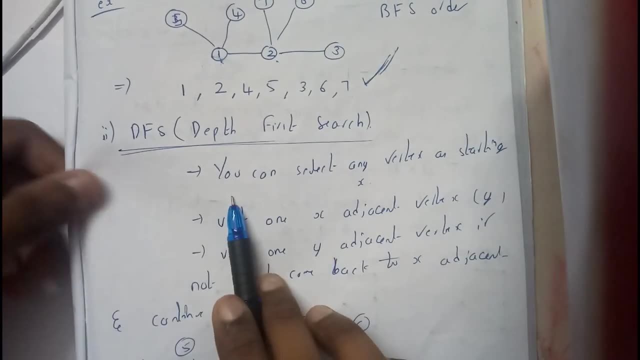 This is a bit complex than the previous. This will be a bit easy, but steps may be confusing. steps may be a bit confusing. Okay, that's fine, I will be teaching you in the best way. You can select any vertex as a starting vertex. 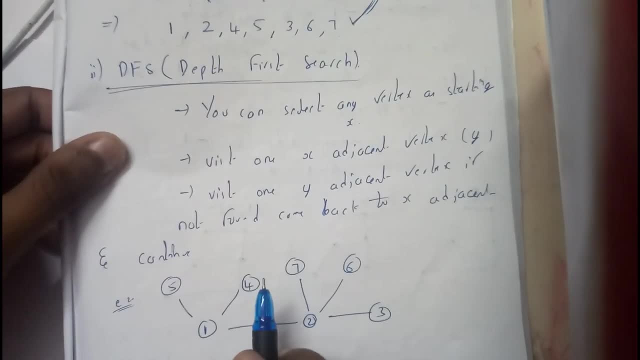 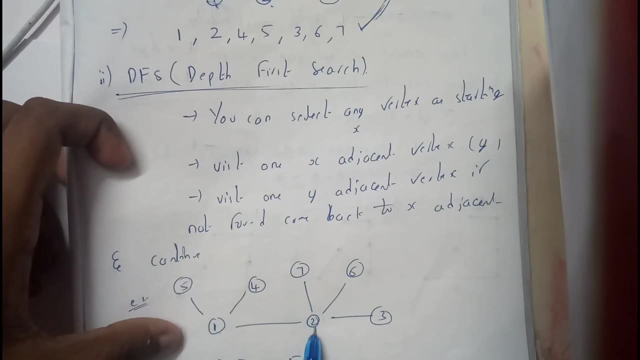 I assumed that. okay, let's take from this better than x and y. Let 1 be the starting vertex, such that 2 is the adjacent vertex, the least adjacent vertex. From 2 move on to 3, the next adjacent vertex. 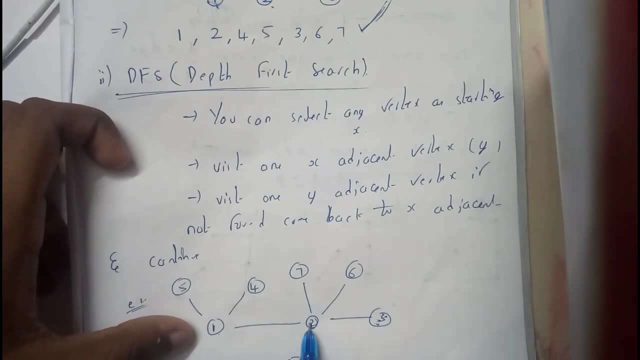 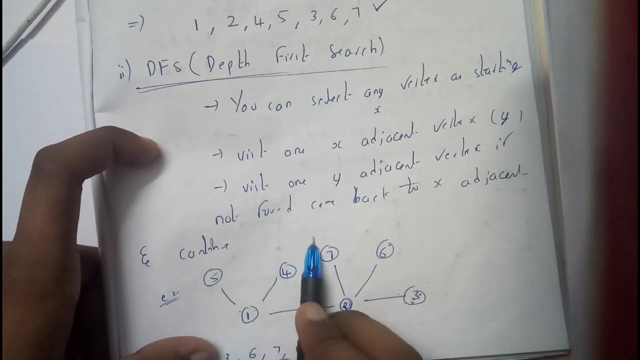 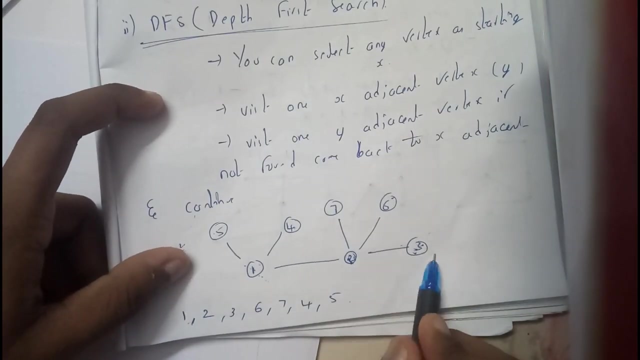 And from 2 move on to 3,, the next adjacent vertex. From 2, move on to 3,, the next adjacent vertex From 3. there is no adjacent vertex, so return back to 2, for 2, 6, from 6: there is no adjacent, so return back to 2, 2, 7, 7,, no adjacent. return back to 2, for 2,. all are done. return back to 1, for 1,. 4, 4,- no adjacent. return back to 1, 1, 5,, no adjacent. that's it: 1,, 2,, 3, 6,, 7,, 4, 5..